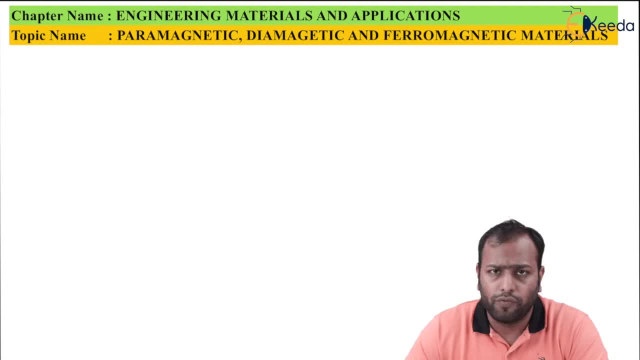 Now, after the discovery of new materials, we came up with a new type of classification that says an alternative theory was introduced wherein solids were divided into two broad groups based on their magnetic dipole moments. So initially a classification was based on mu r or the relative. 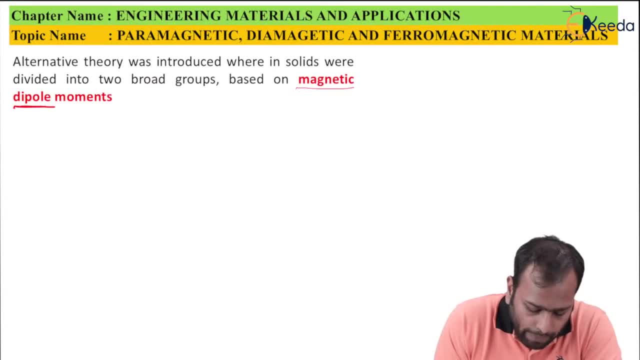 permeability. Now it is based on magnetic dipole moments. Fun fact, it is the most important and the latest classification of magnetic materials. So in exams, so whenever the examiner asks you, state the types of classification. so you need to mention both of this classification. 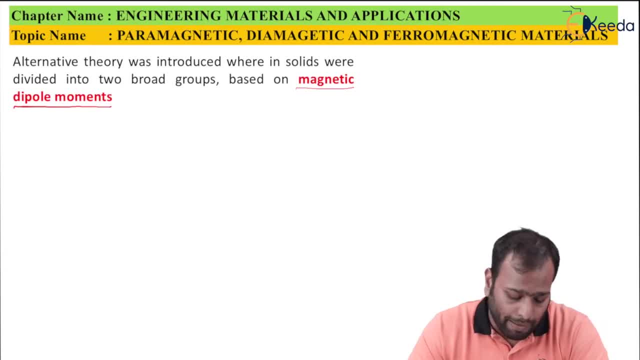 with a light on this topic, that the magnetic dipole moments parameter for classification of magnetic materials is the most latest one Now. so based on the magnetic dipole moments we have when permanent magnetic dipole moment is absent and when permanent magnetic dipole moment is present. So basically based on the magnetic dipole. 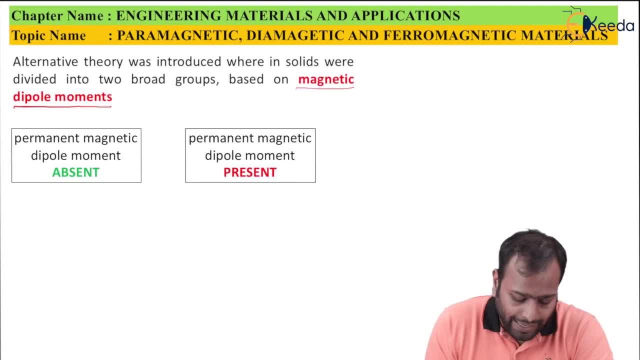 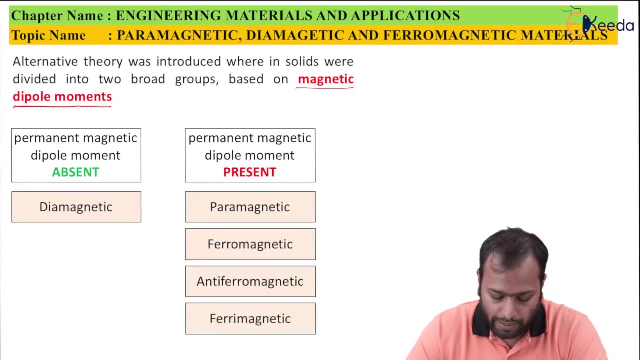 moments. we have two classification: in one it is absent and in second it is present. Now, if it is absent, it is dimagnetic, and if it is present, it is paramagnetic. ferromagnetic- We have anti-ferromagnetic as well as ferry magnetic. So these are basically the subheadings. 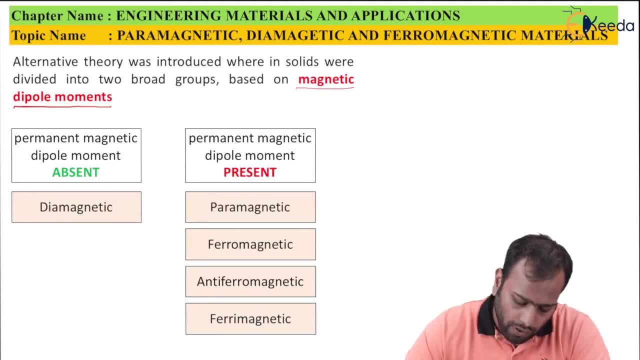 of the classification. Now a point would come. if permanent magnetic dipole moment is absent or present, it is easy to determine: Yes, it is diamagnetic. So how come we can have this four classification? So on what parameter the materials are classified as paramagnetic, ferrimagnetic, antiferromagnetic. 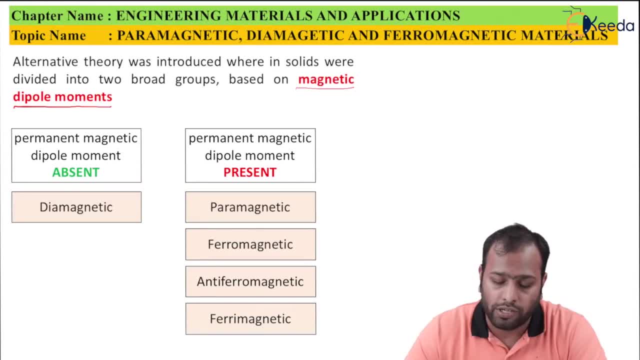 and ferrimagnetic. So well this classification is done on interaction between the atomic magnetic dipoles, will be looking in details of how this interaction between the magnetic dipole works and how are they classified as paramagnetic, ferromagnetic, antiferromagnetic and ferrimagnetic materials. 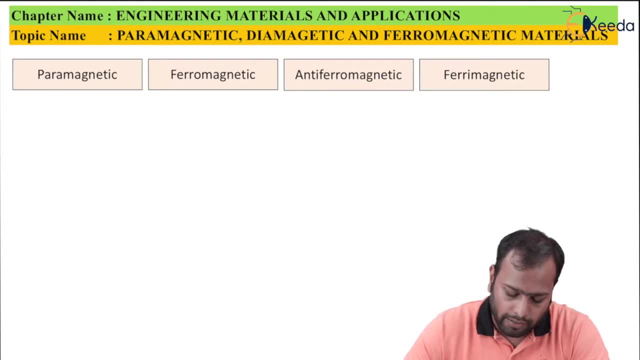 Now let's recall this and see the arrangement in paramagnetic. You can see all the dipole moment. The elements are random, So, in short, they do not follow any trend. However, in ferromagnetic they all are aligned in same given direction. 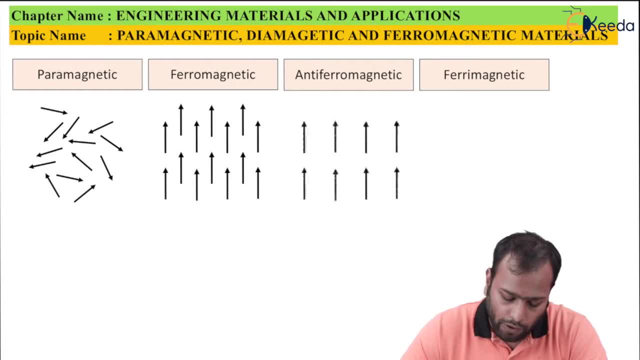 Now what happens in antiferromagnetic? If you see an antiferromagnetic, these are the lines which are same as ferromagnetic, but their neighbors are in opposite direction. Very important transition. You need to notice that the neighbors are opposite in orientation. 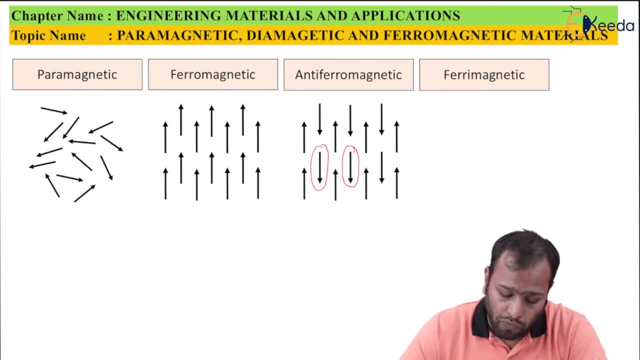 As you can see here. Now, what happens in ferrimagnetic? Well, this is the same as antiferromagnetic with respect to the initial lines, But in the next state the neighbors have opposite polarity. But other than opposite polarity, they also have smaller magnitude. 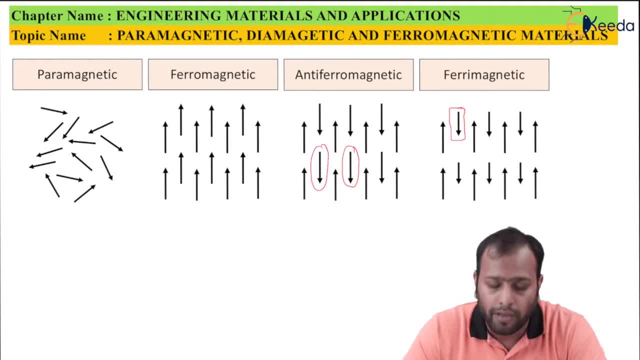 If you can compare The magnitude of antiferromagnetic and ferrimagnetic for the opposite poles, you'll see the ferrimagnetic has lesser magnitude as compared to antiferromagnetic. So this is the most crucial point and important point of classification between antiferromagnetic. 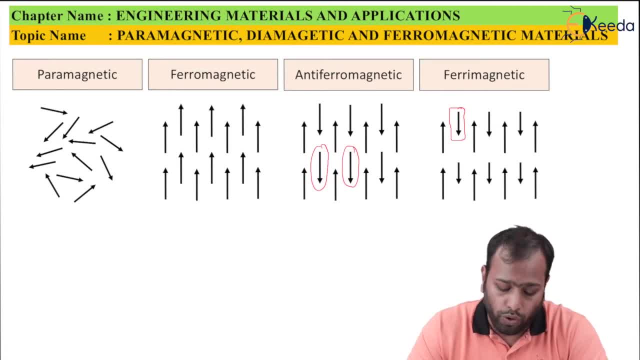 and ferrimagnetic Examiner may ask you to draw the dipoles for antiferromagnetic and ferrimagnetic. So whenever you are drawing for antiferromagnetic you need to make sure that both of the lines should be approximately of the same size. 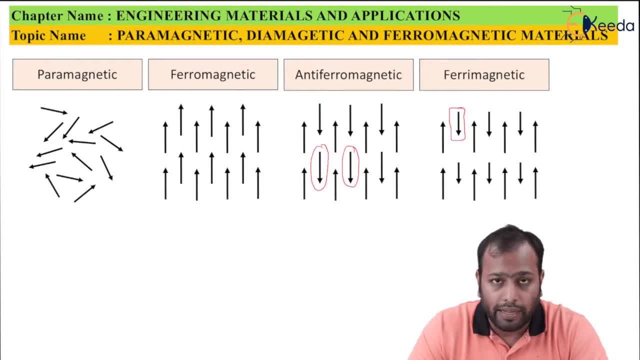 Whereas in the case of ferrimagnetic, your lines in the neighbor which is pointing opposite should be smaller than what is pointing in the forward direction. So this is the most important critical point in ferrimagnetic materials. Now let's take the most important and the crux of this chapter, that is, the distinguish. 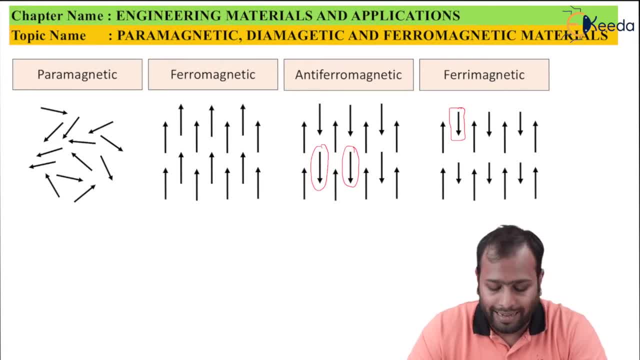 between the paramagnetic, ferromagnetic and diamagnetic substances. Do remember that this is the most important Question for your university exams, which is asked for around 5 to 6 months, So make sure you write down at least 8 to 10 points in that. 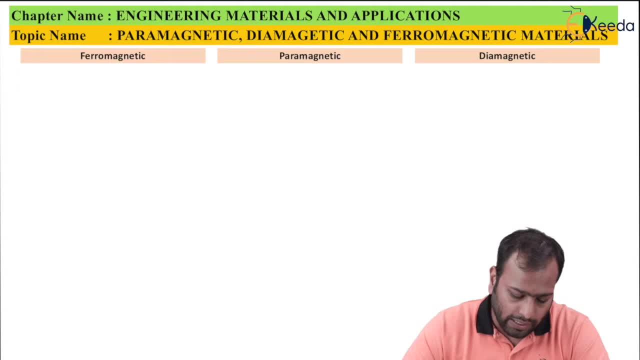 So let's begin Now. we'll take three types of materials: ferromagnetic materials, paramagnetic materials and diamagnetic materials. The first point is: ferromagnetic substances are strongly attracted towards magnetic field. Paramagnetic are feeble attraction towards magnetic field and diamagnetic substance shows 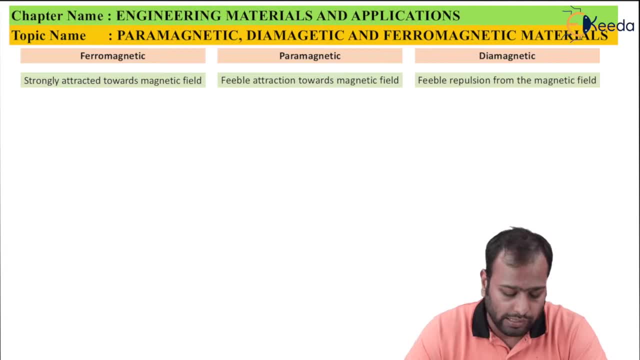 feeble repulsion from the magnetic field. As you can see, the ferromagnetic are strongly attracted. paramagnetic shows feeble attraction, whereas diamagnetic show feeble repulsion to the magnetic field. Second point says field lines are concentrated in the material for ferromagnetic. 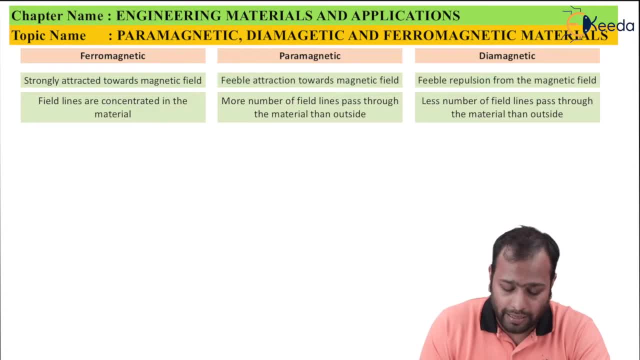 For paramagnetic it says more number of field lines pass through the material than outside. As you can see, the paramagnetic materials has field line passing through the material. The field lines are concentrated in the material, The field lines passing through the material as well as outside. 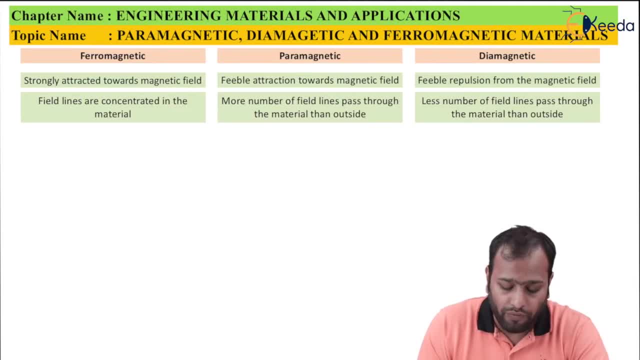 But yes, it is make sure that more number of field lines pass through the material than outside. However, in diamagnetic, less number of field lines pass through the material than outside. In paramagnetic and diamagnetic, this is the most important classification. In paramagnetic, more field lines pass through it and in diamagnetic, less field lines pass. 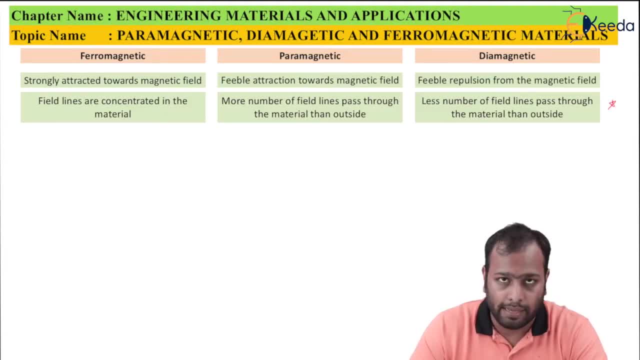 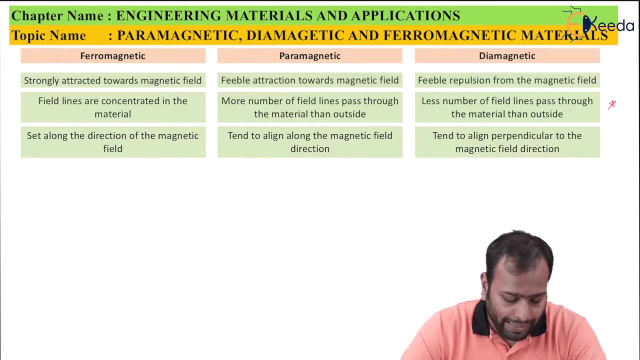 through it Again. this point is a crucial point for your YY exams as well. 3rd point says: in ferromagnetic set, the longer the direction of the magnetic field In paramagnetic align towards the direction of the magnetic field and in diamagnetic they tend to be perpendicular to the magnetic field direction. 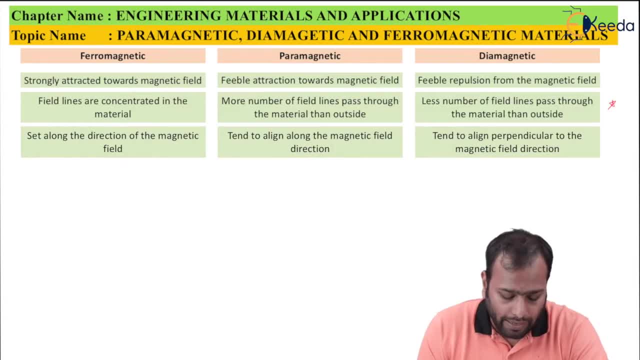 In ferromagnetic magnetic field lines and the poles will try to align them to each other. In paramagnetic they will tend to align them, but it may or mean not not. however, in diamagnetic it will try not to oppose it, but to remain perpendicular to it. 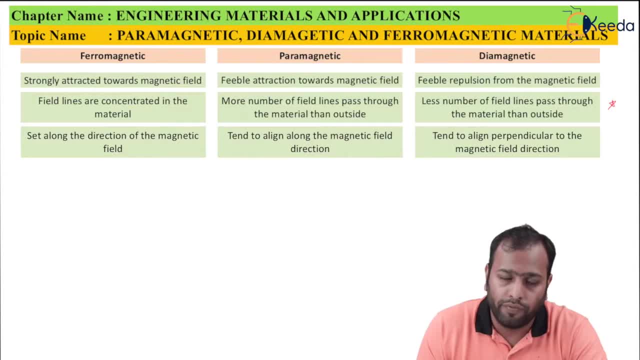 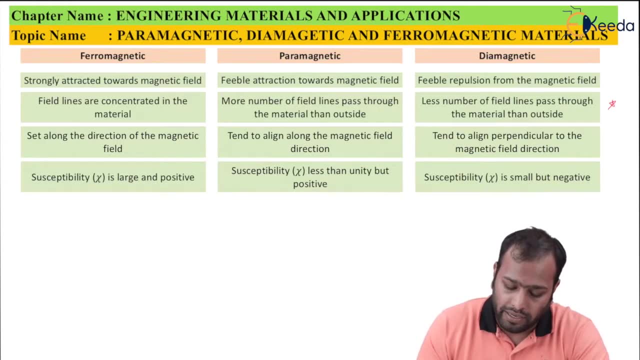 so that the effect of the external magnetic field is minimized. susceptibility is less than unity, but positive for paramagnetic. however, in diamagnetic the susceptibility is negative. so important point: for ferromagnetic susceptibility is large and positive. in paramagnetic it is less than unity, but positive it's only for diamagnetic where the susceptibility is negative. 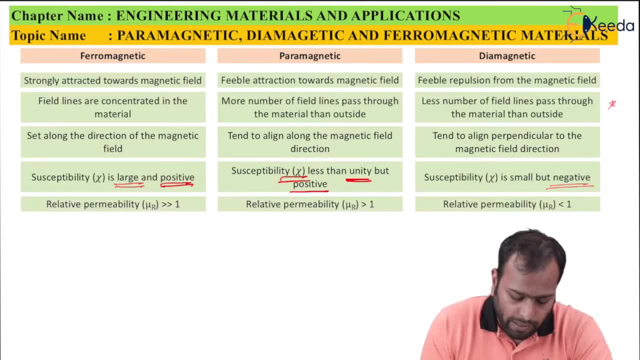 relative permeability mu are much, much greater than one, which becomes for ferromagnetic relative permeability greater than one for paramagnetic and relative permeability less than one for diamagnetic. again, this becomes the most important point because, as discussed earlier, this is the foundation stone for the classification of ferromagnetic, paramagnetic and diamagnetic. 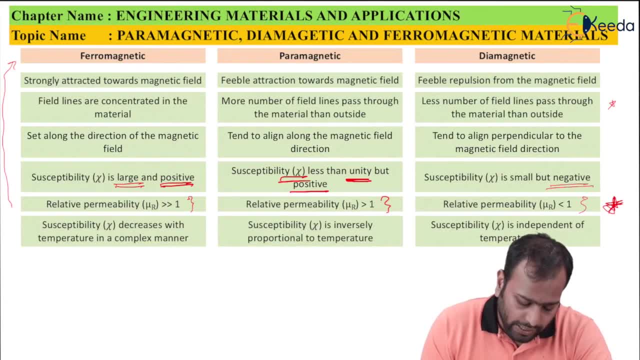 materials. next point says susceptibility decreases with temperature in a complex manner. in ferromagnetic it is known that the susceptibility decreases with temperature, but the manner is complex, which means the manner cannot be quantified or you cannot have a quantitative analysis on which is the pattern in which the susceptibility and the temperature is dependent. 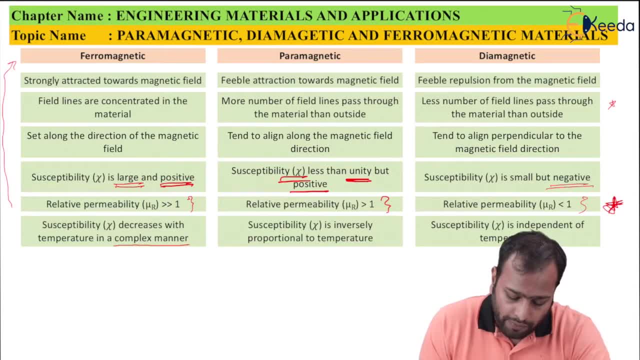 however, in case of paramagnetic, we say susceptibility is inversely proportional to temperature, which is nothing but is the curie's law. you say that susceptibility is inversely proportional to temperature. however, in diamagnetic it is independent of the temperature. so susceptibility has no role to play with respect to temperature in a diamagnetic substance. 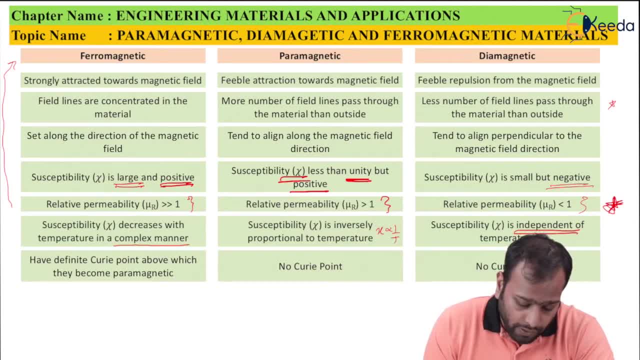 thus we we have for ferromagnetic. those materials have a definite cutie point, above which they become paramagnetic. so we can say: that's a particular point in ferromagnetism material. there is a particular point in ferromagnetic materials, causing which they turn to be a paramagnetic material. so this is the fine. 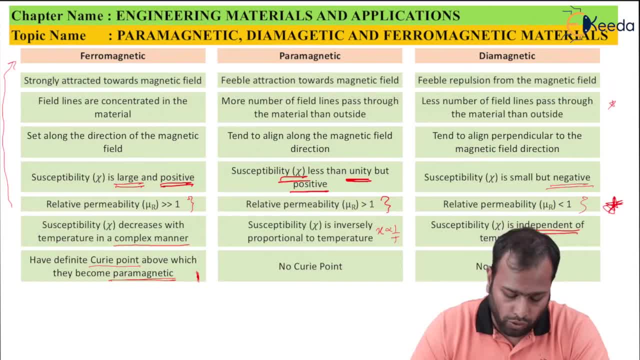 point, which is also known as the floury point. so after this, of ferromagnetic nature, will lose their properties and turn into a paramagnetic material or starts to showing the paramagnet is property. however, in paramagnetic and diamagnetic there is no such Curie point, as well as diamagnetic that there is no Curie point in both of them. next point says B. 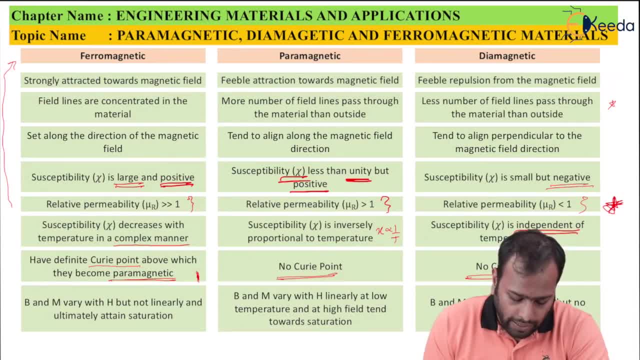 and M vary with H, but not linearly, and ultimately attained saturation. we have studied the relation between B, M and H in the previous class, so this relationship is not linear in terms of ferromagnetic. however, in paramagnetic, B and M vary with H linearly at low temperature and